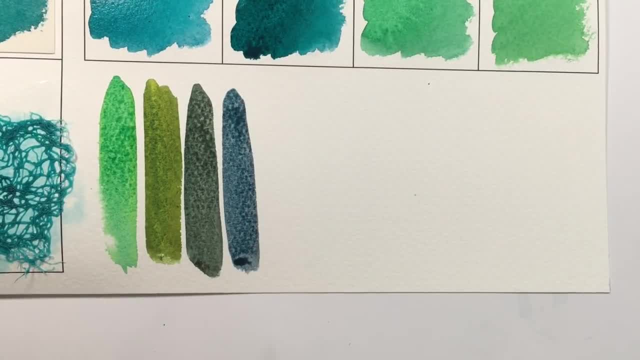 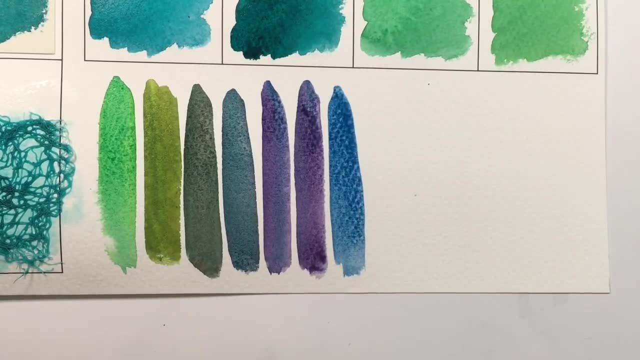 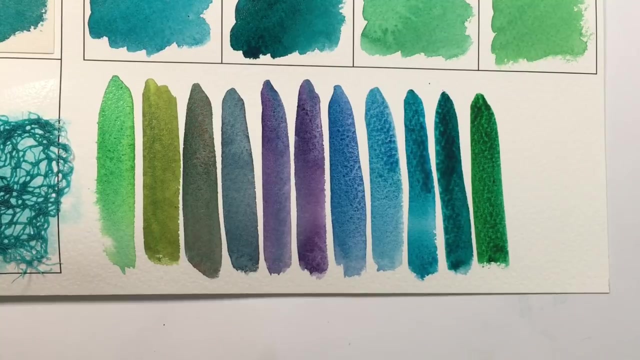 is a deep dirk turquoise that softens into a robin's egg blue when in a single wash. This product is incredibly versatile and can be used for tasks as varied as skies to flowers. It is classified as excellent: light, fast, transparent, not granulating and very staining. 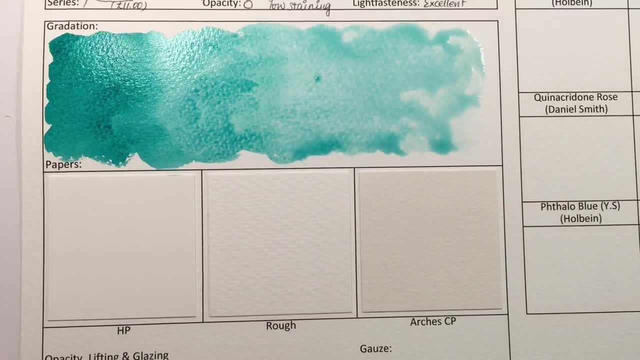 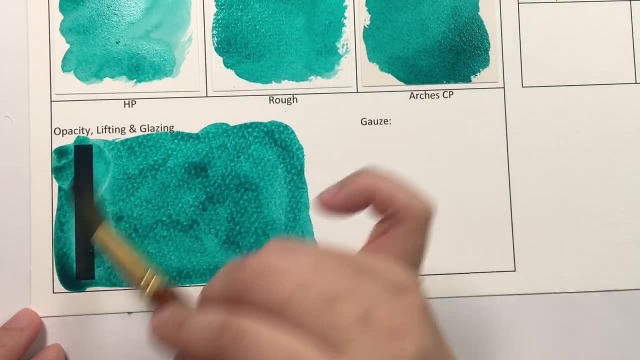 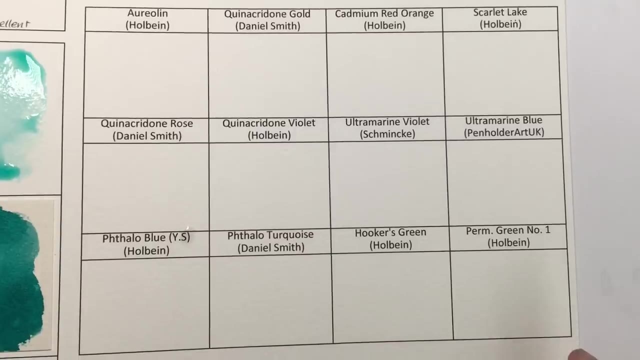 Next up is Ultramarine Turquoise by Daniel Smith. It is a combination of PB29, which is sodium aluminium sulphosilicate, which is your ultramarine blue, and PG7, which is chlorinated copper phthalocyanide, which is your phthalo green blue shade. It is again a series one. This color is a granular. 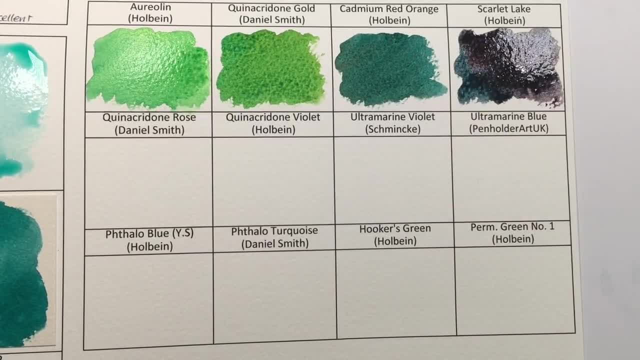 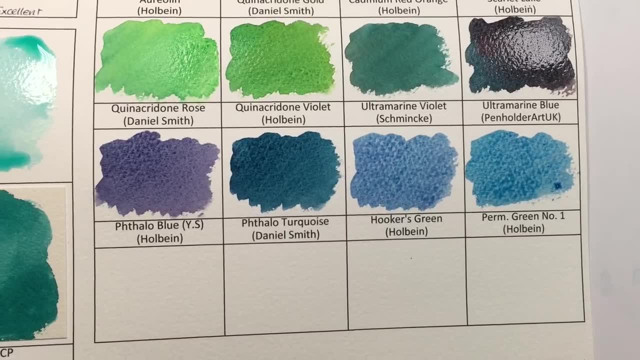 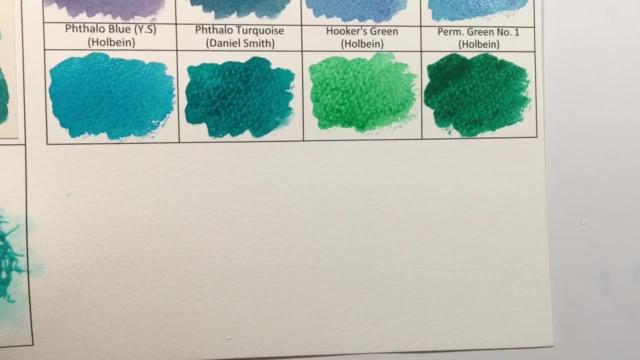 lone staining equivalent of phthalo turquoise and can be used to create unusual grainy washes. It is classified as excellent: light, fast, transparent, granulating and low staining. It also quotes the artist Jean Haines. My new favorite and must have color is Ultramarine. 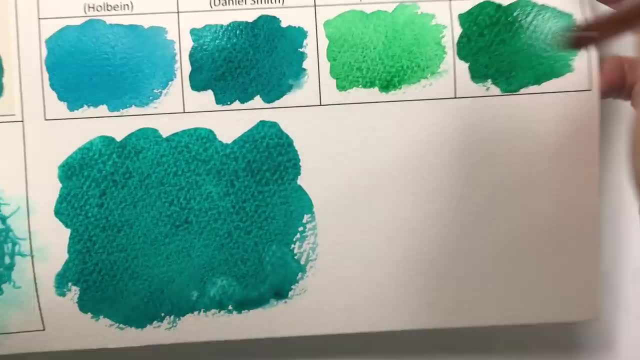 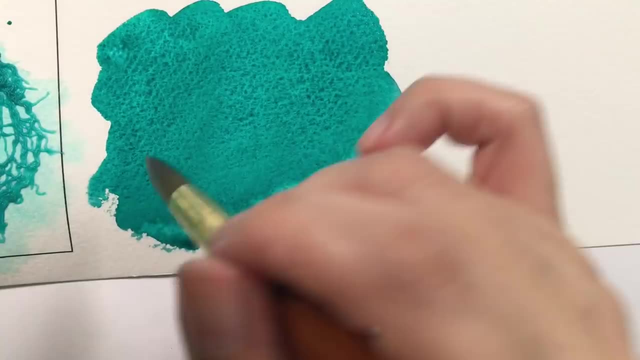 Turquoise by Daniel Smith. It is so vibrant, it creates incredible patterned effects and I love moving freely by the addition of water drops. Do treat yourself to this fabulous shade if you don't already have it. It is amazing. A feel, good color. It is a combination. 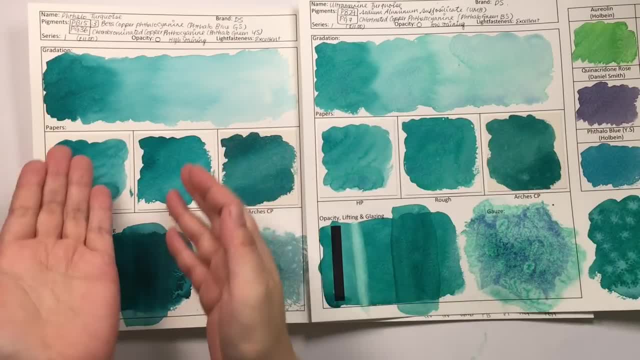 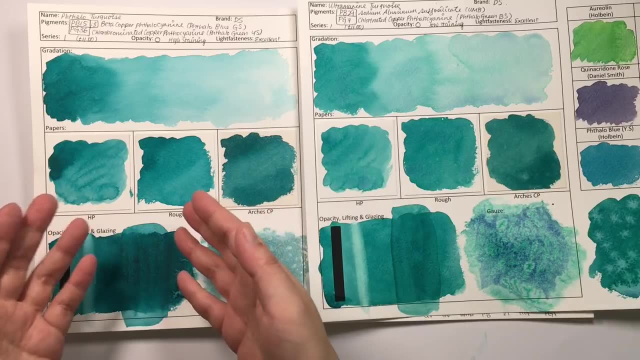 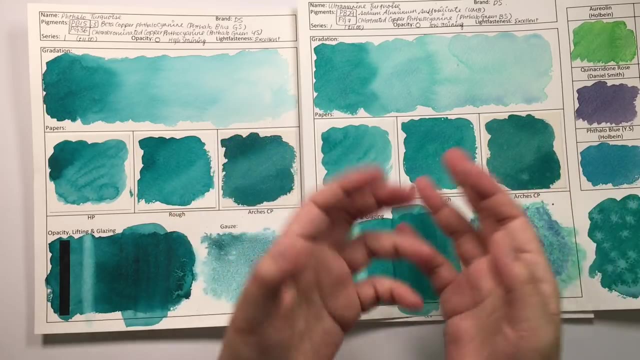 to work with. We're back and the paints have dried. This is phthalo turquoise and this is ultramarine turquoise. First impression in general is that phthalo turquoise is a deeper, more richer, more intense color than the ultramarine turquoise. Ultramarine turquoise has a much softer but 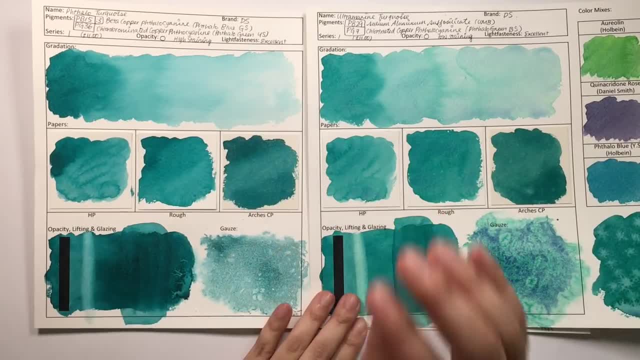 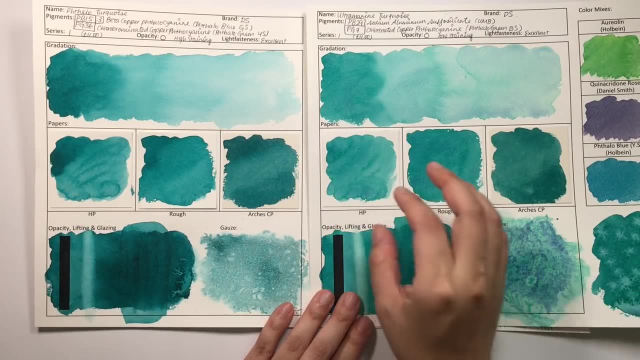 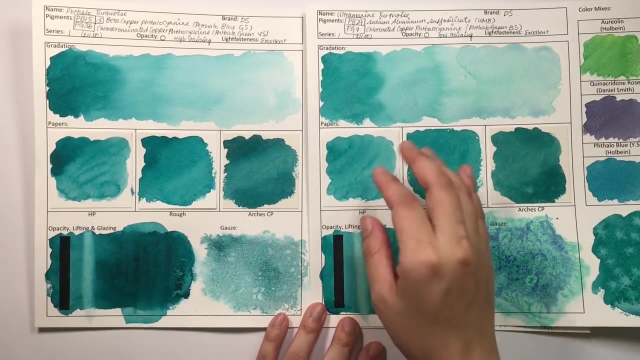 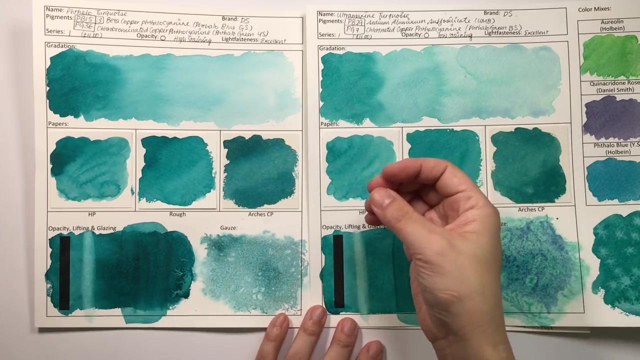 still very beautiful and rich color. What has been a surprise to me personally is that the ultramarine turquoise hasn't granulated much for a color that has ultramarine blue in it. Most other paints with ultramarine blue tends to granulate quite heavily, such as the Rose of Ultramarine and the Imperial Purple. 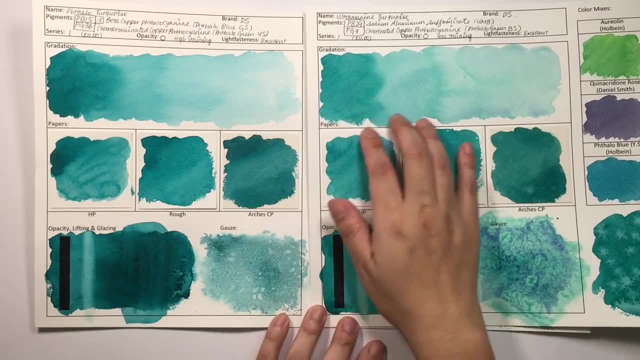 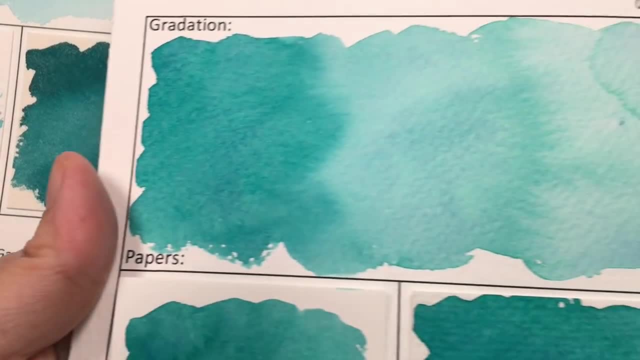 that we tried in Episode 3.. Whereas here it's a lot more subtle, if at all, granulating. Looking at it closer, there are some. there are definitely some granulating. I'm going to take a look at this one. 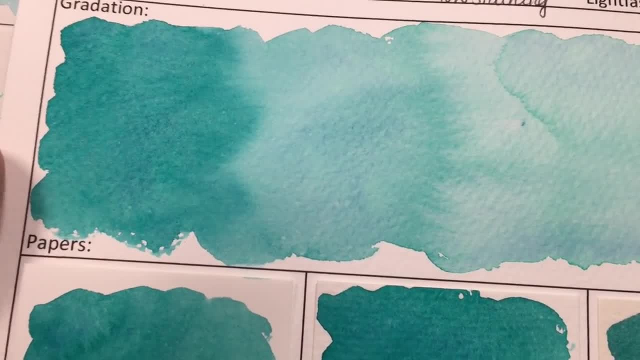 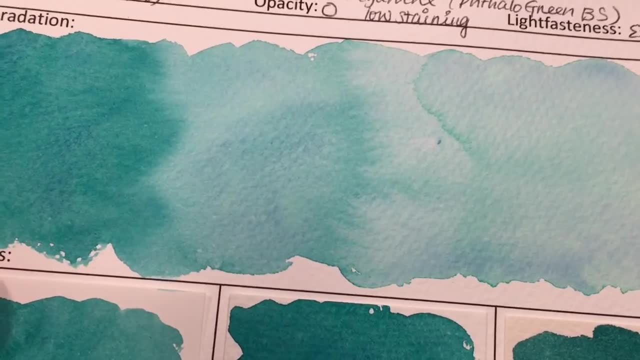 I'm going to take a look at this one. I'm going to take a look at this one. It's very, very subtle. It's a little bit more granulating, but it's very, very subtle. I would say this is comparable to, or even less granulation than, the Undersea Green. that. 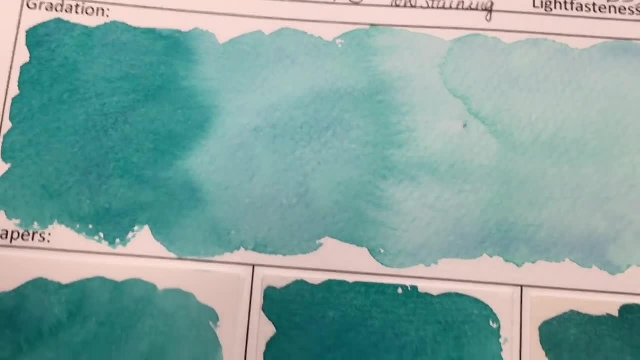 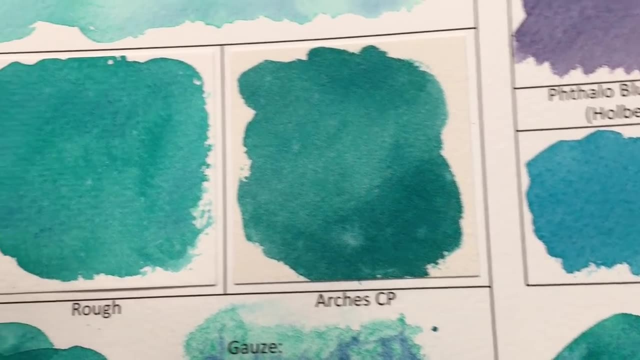 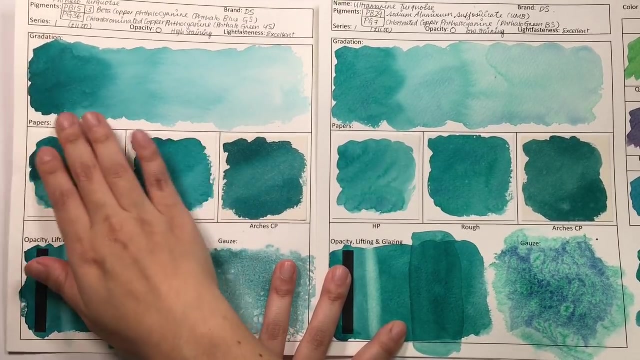 we tried in Episode 2, which for a color that has the name ultramarine in its color name. it's surprising to me of how lately ultramarine it is Now degradated wash. obviously with the phthalo turquoise you get a lovely smooth wash With. 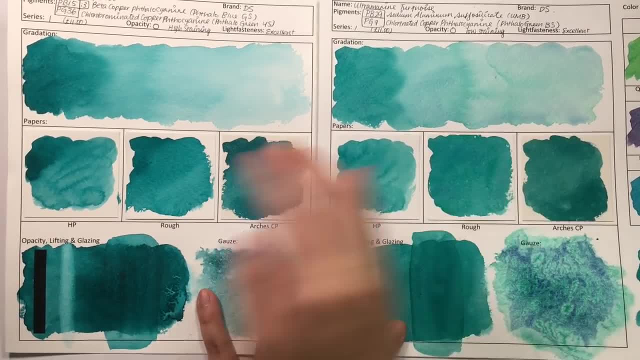 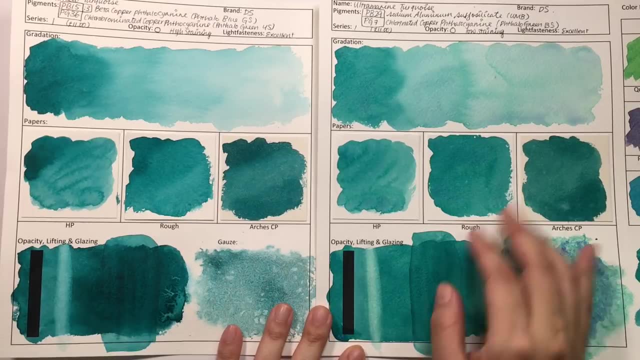 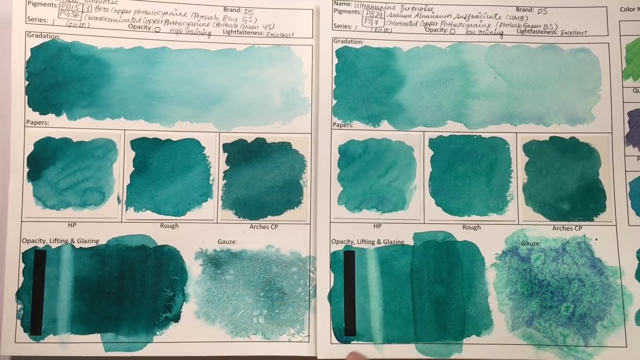 ultramarine. you do get a little bit more texture, but not that much and same with the different papers: pretty smooth overall and pretty smooth overall, with a much darker wash here and a more tealy wash here. in terms of opacity, i would say they are both transparent, lifting wise. yes, the 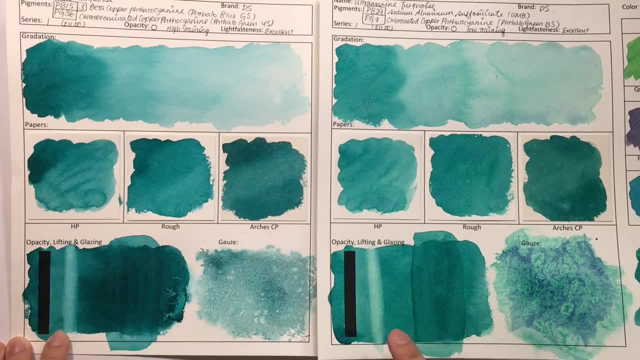 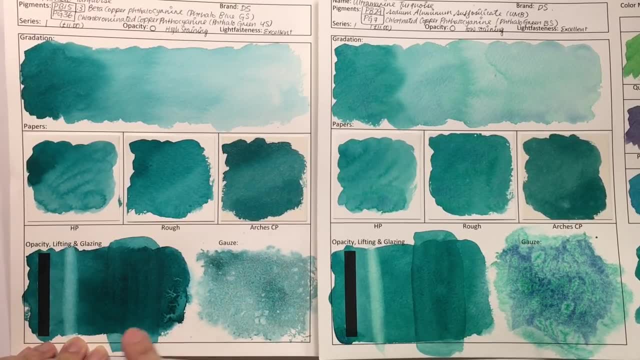 sale of turquoise was a little bit harder to lift than the ultramarine turquoise. now i didn't do a very good job here, but i know thalo turquoise layers beautifully and you can put many layers as you want and it will just keep layering and it's one of my favorite layering colors. 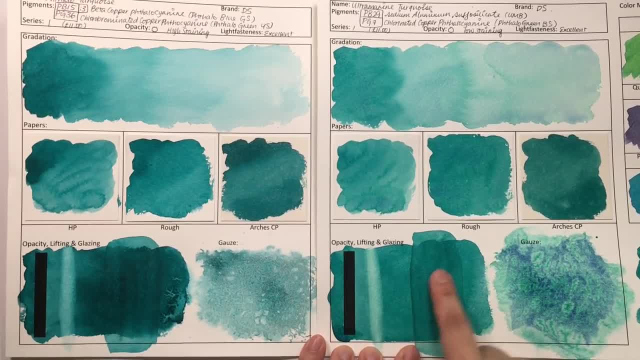 layering ultramarine turquoise will give you a little bit more granulation than you notice in a single layer. so if you want a stronger granulation out of this color, then glazing it is a great idea. what was a surprise was the gauzing, and now i knew that the sale of 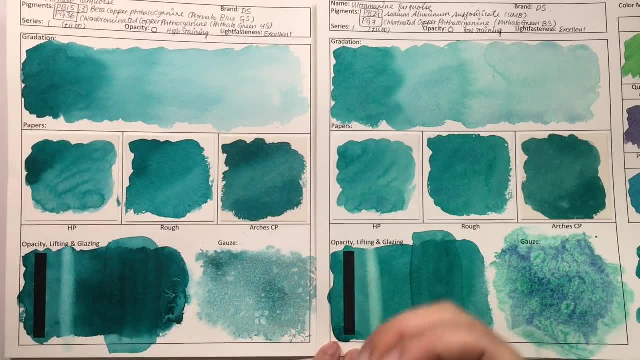 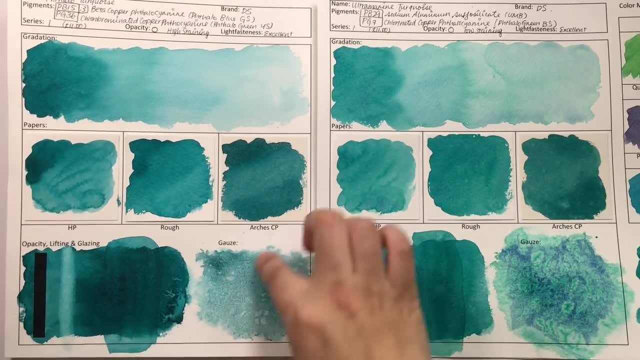 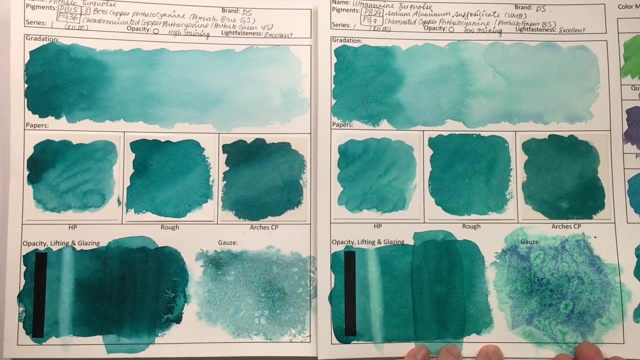 turquoise was going to do this thing, because thalo colors aren't very good at doing gauzes- or they will do this thing where it acts more like a mask than creating the lines that i normally go for. however, pull it off old ultramarine turquoise for a color that has ultramarine, which i know for. 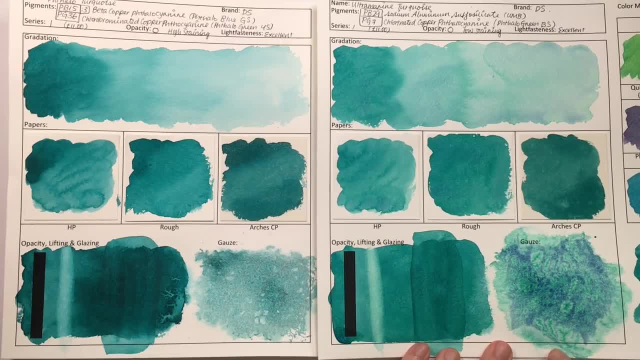 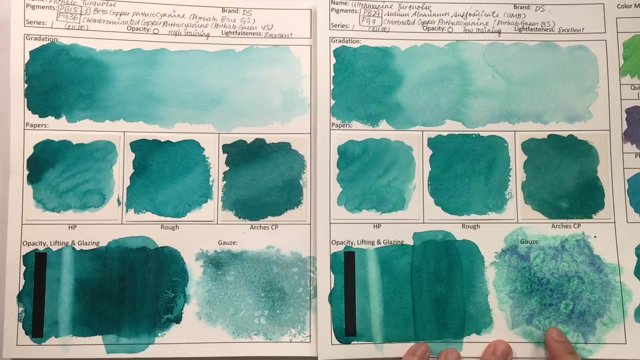 fact is a really strong gauzing color. i was really surprised when i peeled the gauze off on how faint and muddly this was, not impressed might be useful for a particular thing, but in terms of getting really definite lines it's not a good color to do because it seems to have such 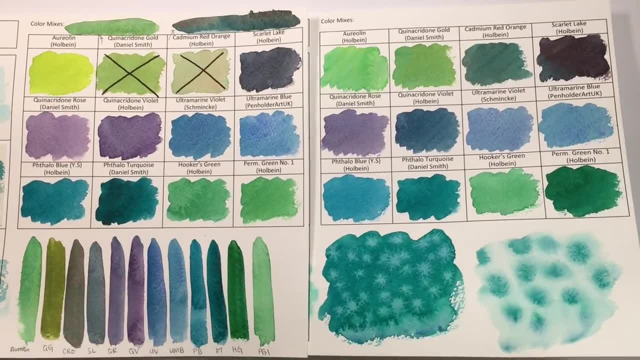 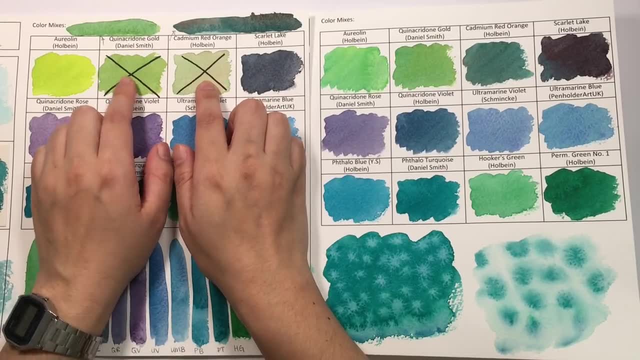 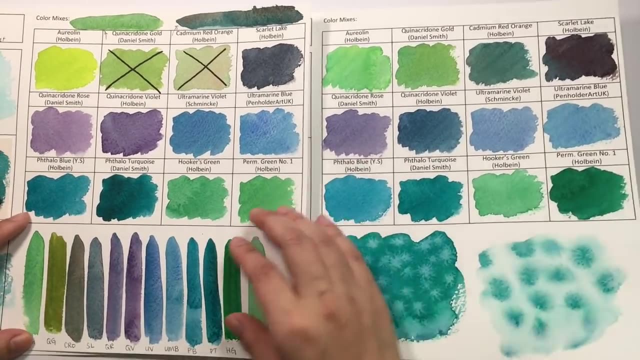 a little amount of the ultramarine in terms of mixing colors. i'm really sorry i messed up these two. i mixed hookers green in it instead of the thalo turquoise, so i've redone it here and just so that you can get a good impression of what the 12 colors look like together, i've redone all 12. 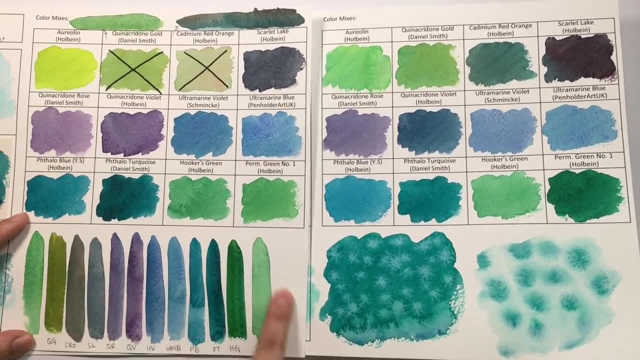 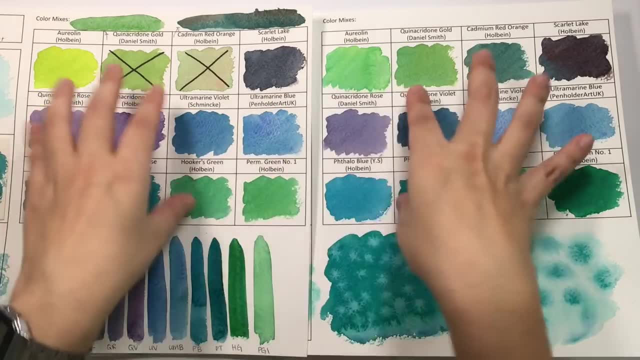 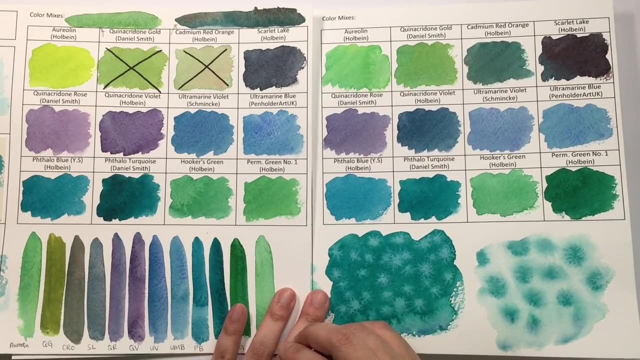 colors here for you so that you can have a good feel as to what thalo turquoise can do to other colors. i would say they're both very, very similar in behavior. in terms of mixing with other colors, there isn't that big a difference between the two in the color produced. the complement of thalo turquoise is scarlet lake in my palette. 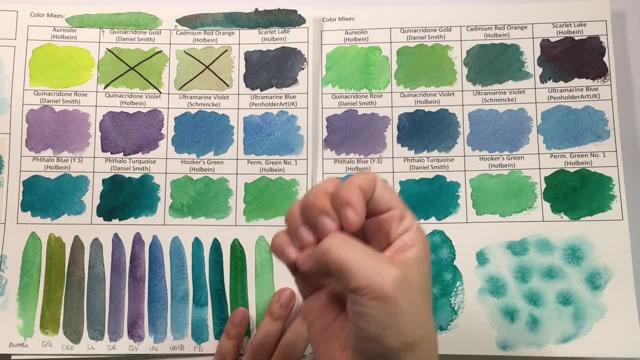 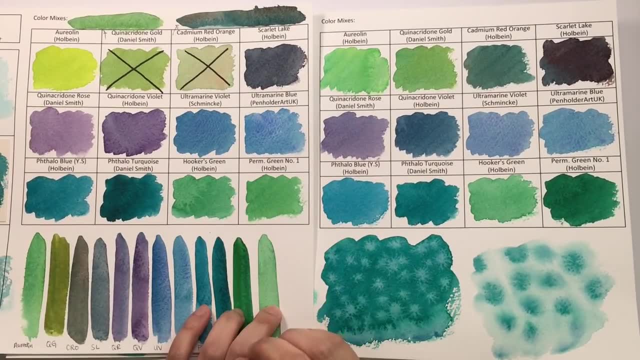 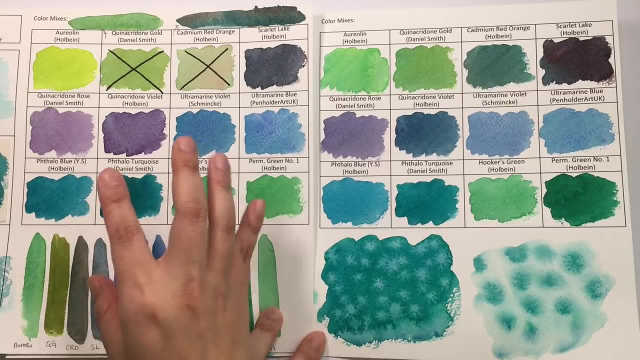 and so they both neutralize quite nicely into this dark inky color and it creates beautiful greens. so overall, in terms of mixing with other colors, they're interchangeable pretty much. i think you might be able to get a slightly darker mix out of the thalo turquoise than the ultramarine turquoise. 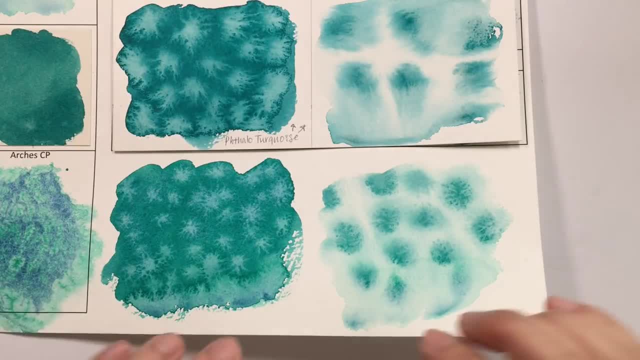 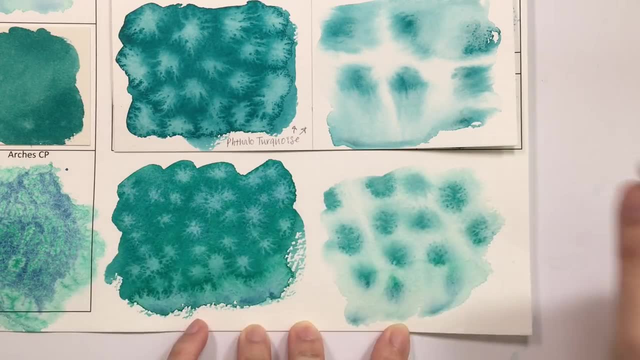 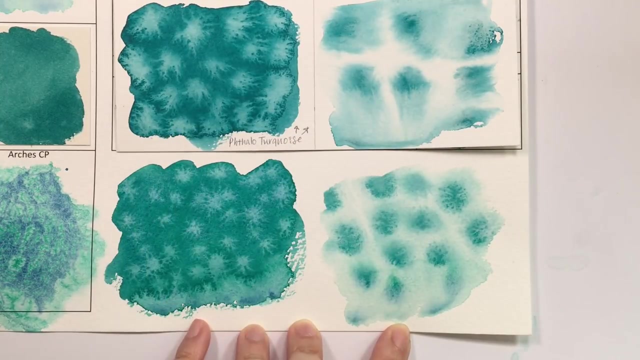 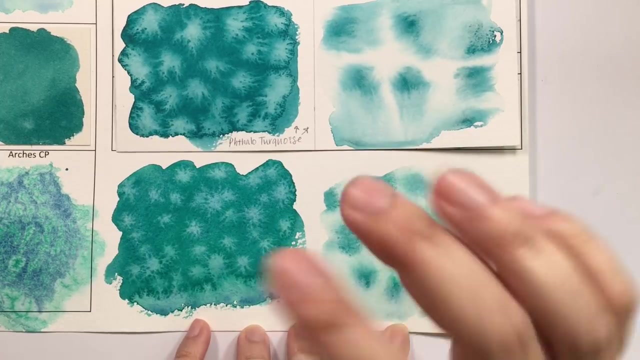 because jackson's website quoted jean hayes saying specifically that the ultramarine turquoise is a great color that moves freely in water, i thought i'd test how well it moves. so this is thalo turquoise and this is ultramarine turquoise. in these two i did a wash of each color, waited a few moments and then dropped. 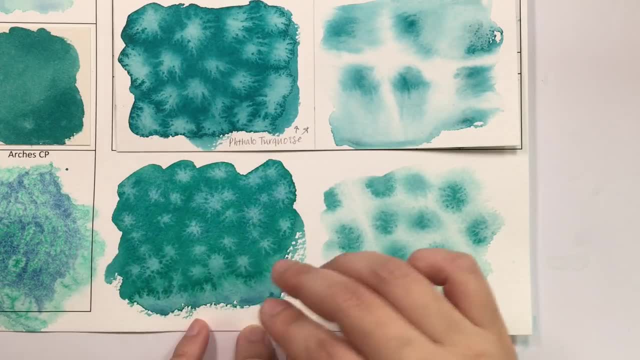 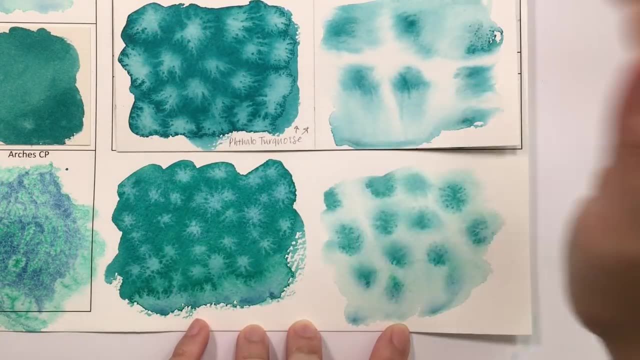 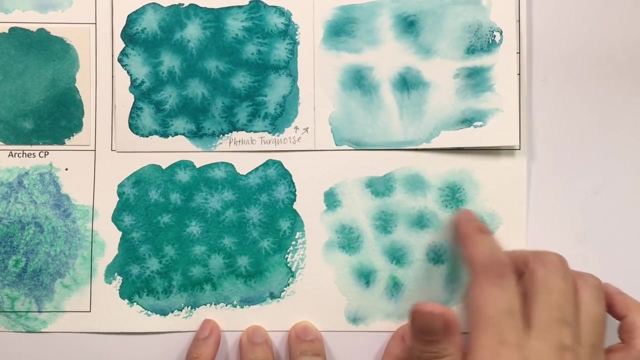 some water onto it to see how water moves within the paint. this side, i did a clear water wash and then dropped some paints in. in terms of the ultramarine turquoise is true, they do move around quite nicely. they they break up into these textures, which are fun. 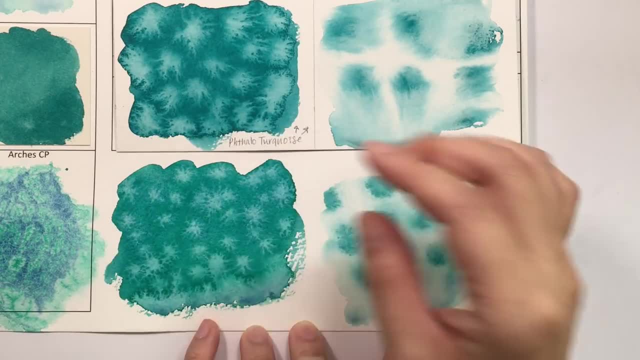 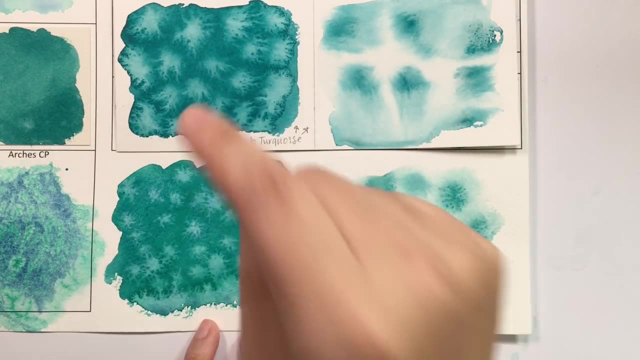 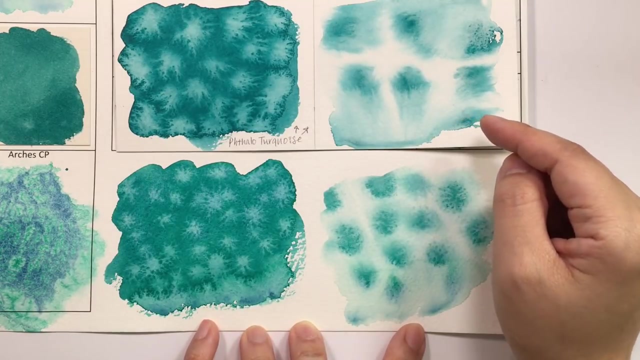 and they also bloom quite well. however, if you want that effect, thalo turquoise is a much better one. the reason why there are fewer dots in the thalo turquoise is that it emits poison. you can see that my sun louis is referring to thalo turquoise, which is me. 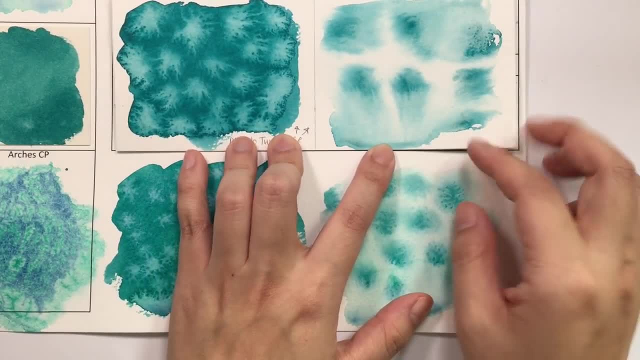 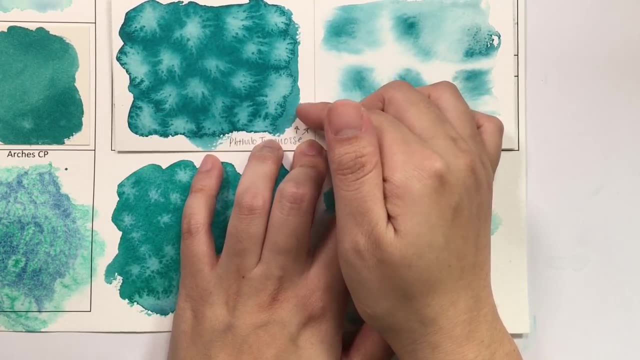 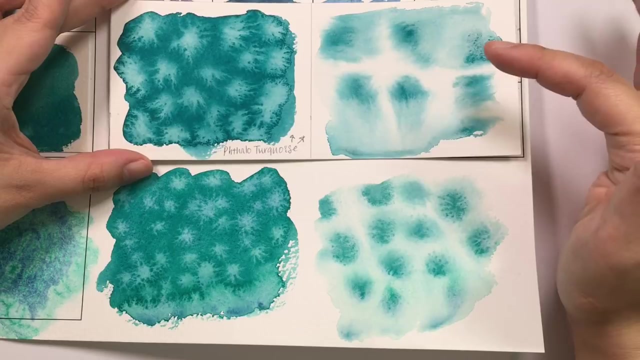 here on the right and i two Danielle bin October. um well, Thaylo is a voluminous vernal. throw it through her skin here, which is why Iáuhed her trich inheritance contract. clear Du 130 dieter. it's fine, I guess, because Thaylo Turquoise does an flaws in my skin- former ones- and then it just runs. 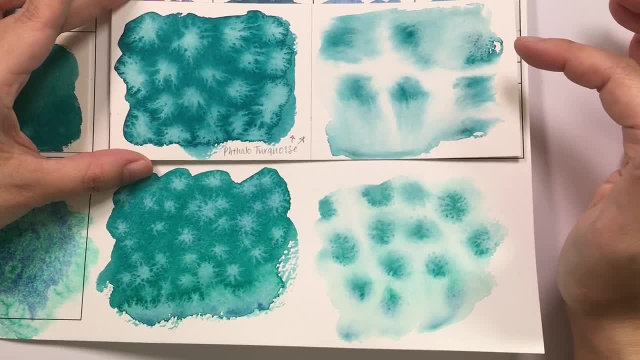 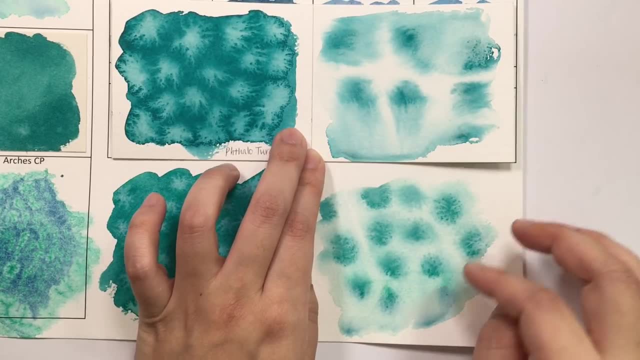 away as the water draws when it does. in that case, then ethelo turquoise. I will get on the other ones too. phthalo turquoise is definitely the paint to go for the only time I would pick ultramarine turquoise over the phthalo turquoise in a. you know this. 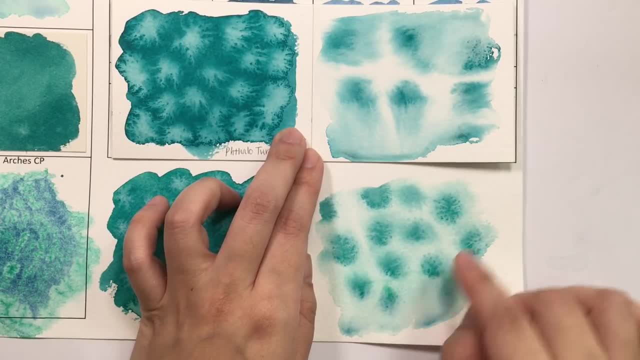 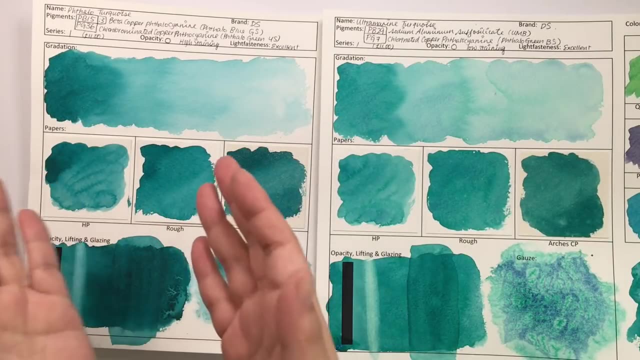 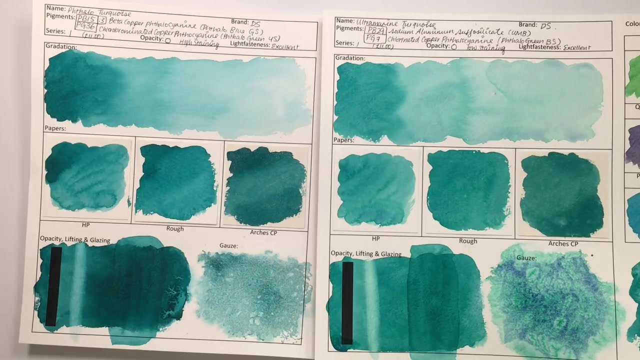 effect is if I specifically want this particular, more broken-up texture. in conclusion, for me personally, phthalo turquoise is still one of my favorite colors. it is beautiful, it does amazing things, whereas the ultramarine turquoise- I have to say it was a little bit of a disappointment for me if ultramarine 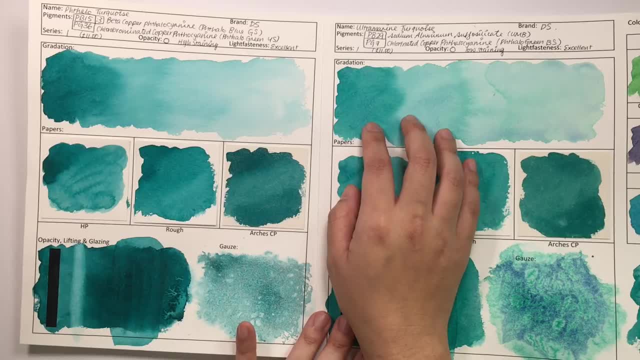 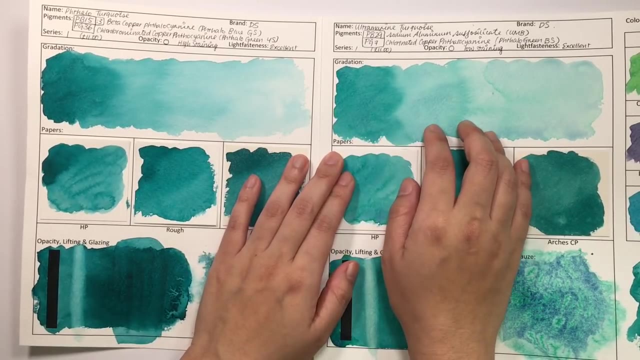 turquoise. had a little bit more ultramarine blue in it, I think it would be a different matter. however, I can also understand where they can't put any more ultramarine blue in it, because then it will be less of a turquoise color. they are a good match to each other, but for this being an alternative color to the 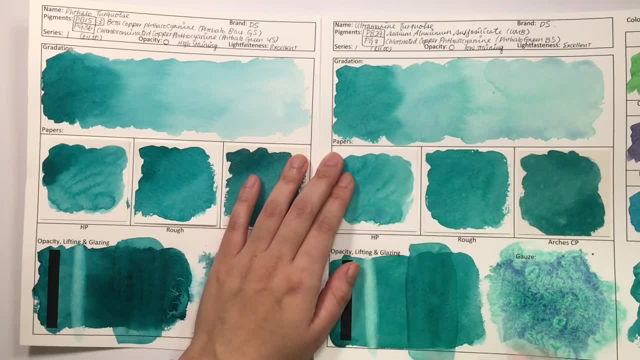 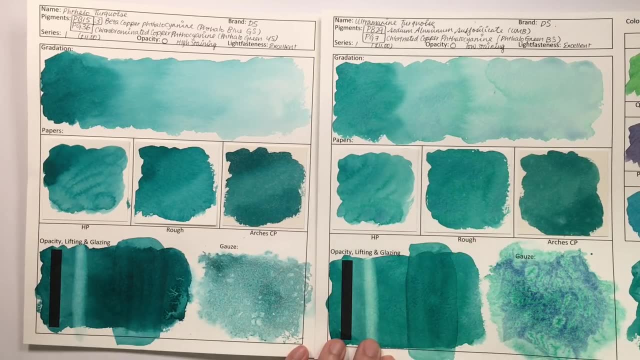 phthalo turquoise. I would pick ultramarine turquoise over the phthalo turquoise in a for when you want granulation. I don't think it does a particularly good job of granulating. if you need ultramarine turquoise to granulate a lot, then your. 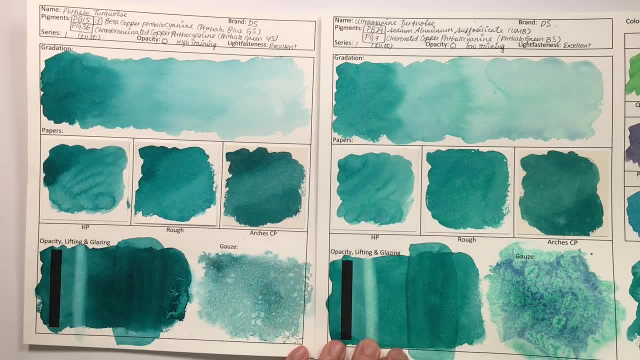 best bet is to layer the paint in at least two layers, because that makes the granulation come up a bit more in terms of causing, unless you're looking for these particular textures in terms of getting really strong defined lines, I don't think either of them are suitable. 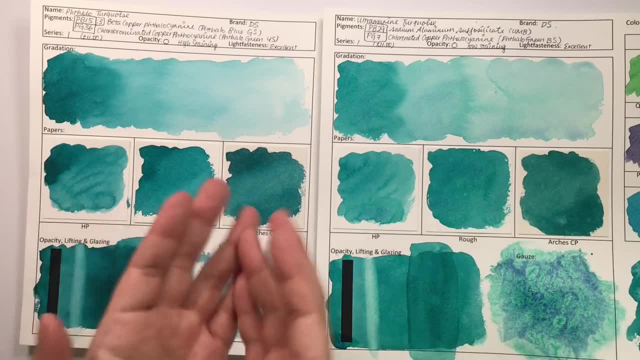 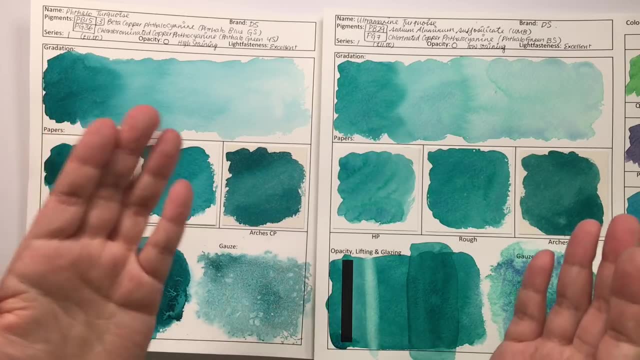 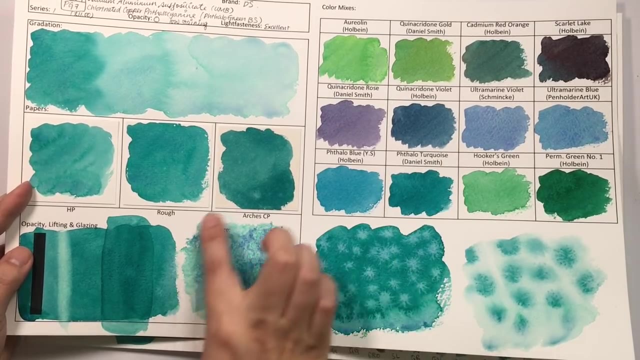 and in terms of mixing colors they are pretty much the same. so for me the phthalo turquoise is definitely staying on my palette and the ultramarine turquoise is probably not gonna make it to my palette. I'm glad I have it for if I ever need this kind of particular texture or this kind of broken-up. 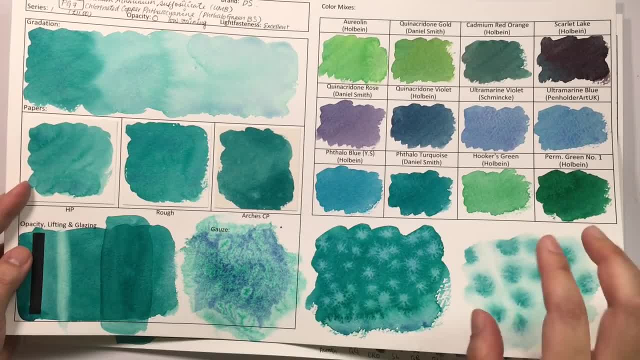 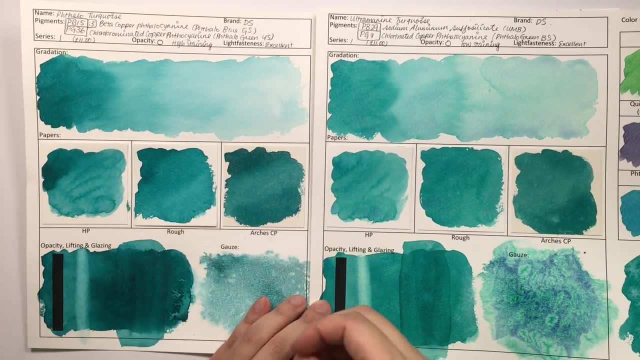 texture you get when you charge the paint into water. but I don't think it will make it into my palette because it that is very, very specific use for the specific use and I'd rather just pull the tube out when I need them. how about you? which one would you pick? would you pick phthalo, turquoise or the Altra?